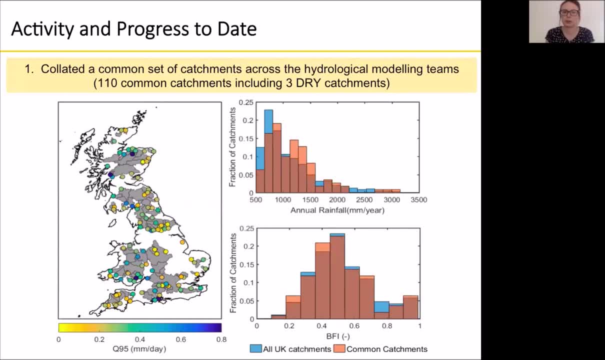 orange is the histogram from our comment in terms of water scarcity, The verbatim zero, which is the concentration rate for of annual rainfall, and the base flow index, ie the proportion of flow that's coming from groundwater sources, And you can see that we're covering quite a wide diversity. 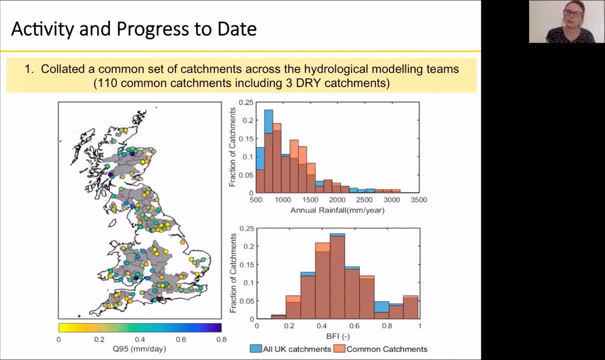 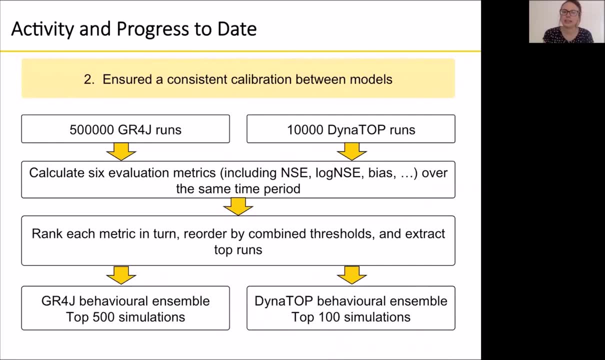 so these catchments essentially are a good representation of catchments across Great Britain. The second thing that we've been doing is ensuring a consistent calibration between the models. So our models are calibrated to provide the best fit to observed flows, And here what we've been doing. 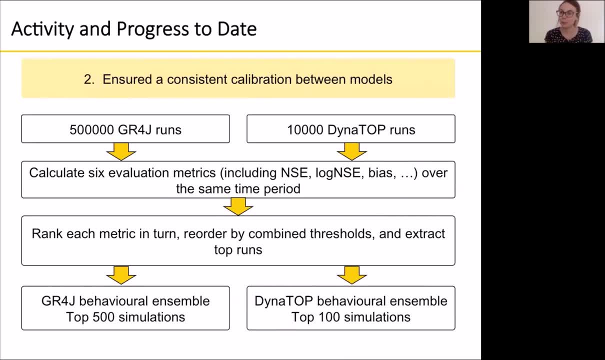 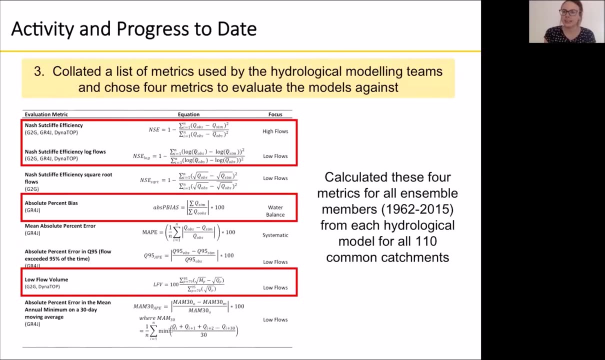 to ensure that our models are as comparable- or our model outputs are comparable- as possible. we've been using exactly the same calibration techniques for two of the models, that's, GR4J and the dynamic top model. Finally, the final thing that we've been doing, 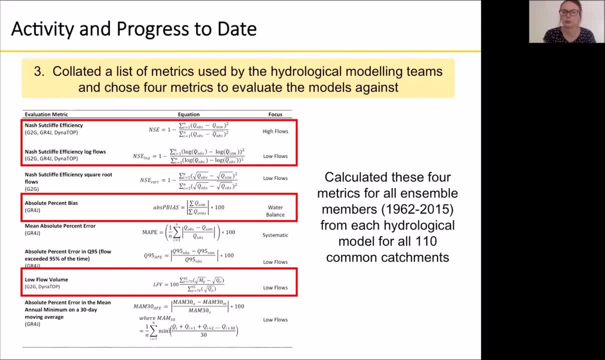 we have collated a list of metrics used by the hydrological modeling teams and chose four models and four metrics to evaluate the models against. So this is a really important part of the hydrological modeling into comparison is: how should we evaluate our models and say how good they are in different catchments? 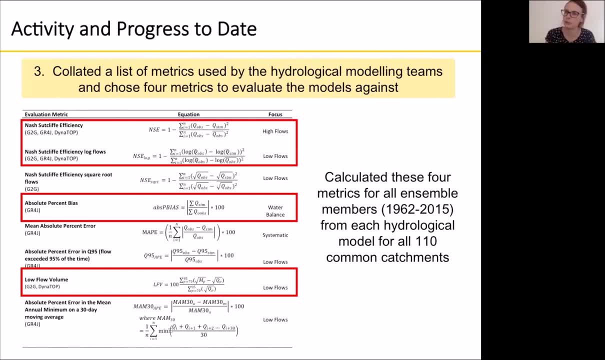 So we collated a massive list of metrics that we'd all evaluated our models against, and then we chose four, essentially, One focused on high flows and more of a common, commonly used hydrological model metric, which is Nash-Sucker- Nash-Succliff efficiency. 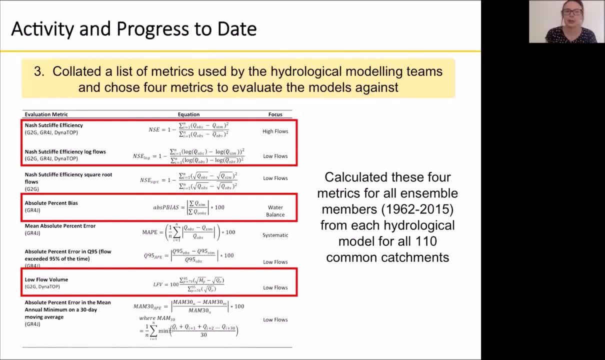 But then obviously we focus more on droughts and low flows. So we also use log Nash-Succliff efficiency absolute percent bias to focus more on the water balance aspects and then the low flow volume as well, which are highlighted in red. 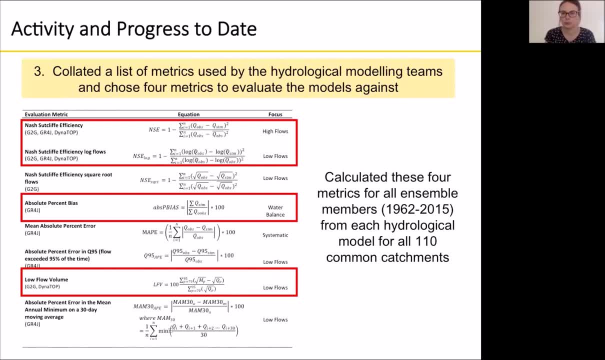 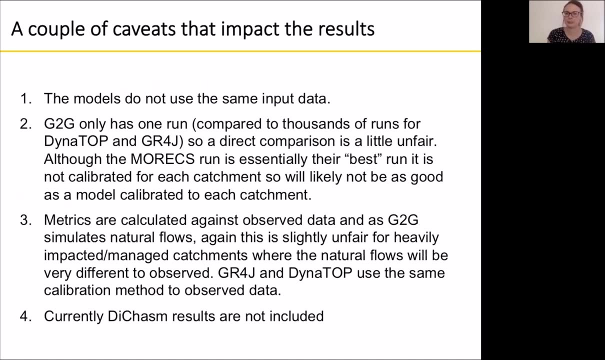 And we calculated these four metrics for all ensemble members from 1962 to 2015,, from each hydrological model for all 110 common catchments. Just a couple of caveats that impact the results that I'm presenting today. Firstly, the models. 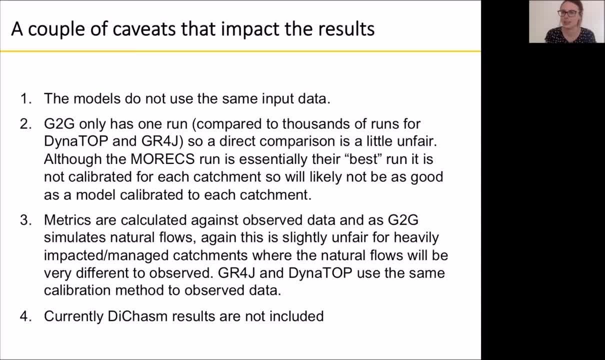 you know, one of the big points of comparison is the models don't actually use the same input data. They use slightly different rainfall products and also quite different potential evapotranspiration products, So that's something that does affect the results. We have three different models. 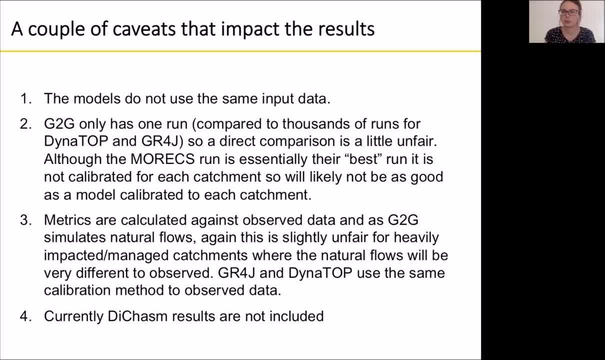 that I'm presenting results from today And grid-to-grid only has one run compared to thousands of rounds for the dynamic top model on GR4J. So a direct comparison that I'm showing you is actually a little bit unfair on grid-to-grid because they only have one simulation to test against. 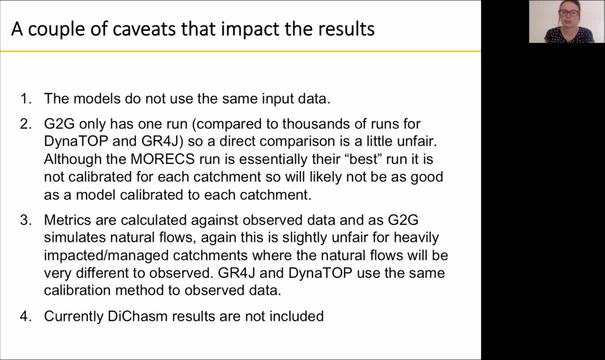 whereas we've directly calibrated two particular output flows. So it's likely that grid-to-grid won't be quite as good as a model calibrated to each catchment, And so the third point is that you know. the third point is that metrics are calculated. 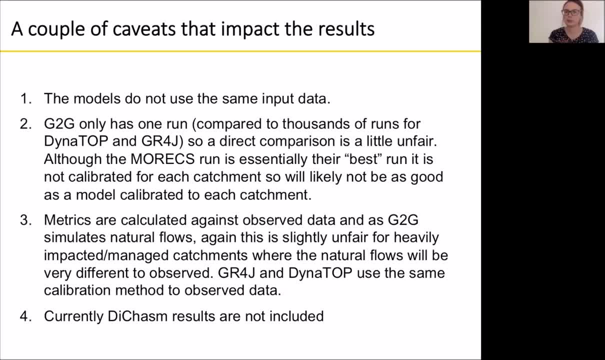 against observed data. Now for dynamic top model and GR4J. we calibrate our model simulations to this observed data to get a reasonable fit to the flow that was observed at the gauge. However, grid-to-grid simulates natural flows, So again the model results will look a little bit different. 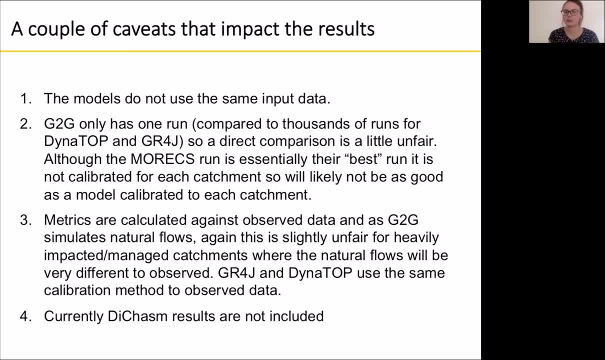 for heavily impacted or managed catchments, where the natural flows will be very different to the observed. Final point is that currently we don't have any results from the DRIVE project, which was also part of the Droughts and Water Scarcity programme. 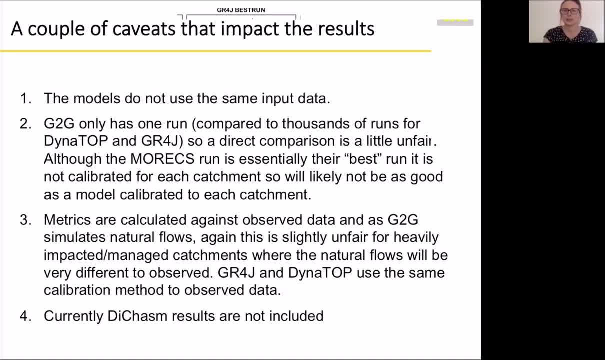 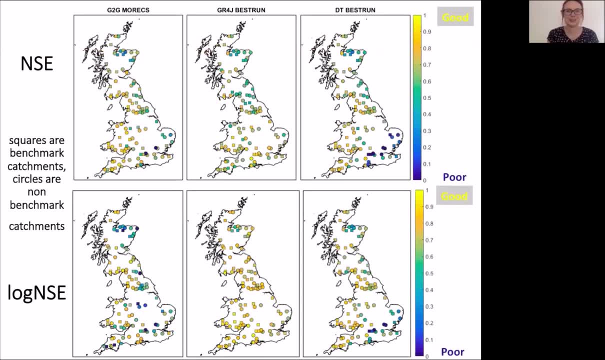 but these will be added in due course. So in terms of the results, this is a very busy slide, but I will talk you through it. And so in the top panel you have Nash-Sutcliffe efficiency. Each point represents a gauge. 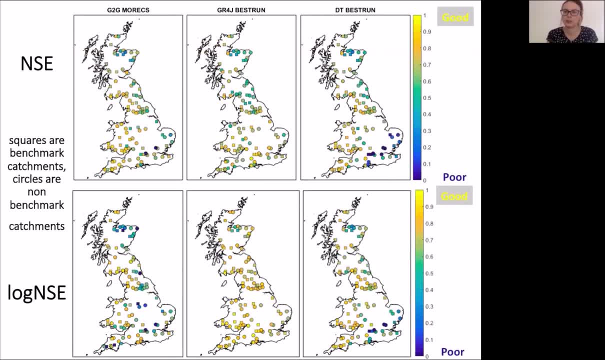 Yellow denotes good model performance, blue denotes poor model performance, And what we've done here is: the squares are benchmark catchments, ie catchments that we believe to be not as heavily impacted by human influences compared to the rest, And the circles are non-benchmark catchments. 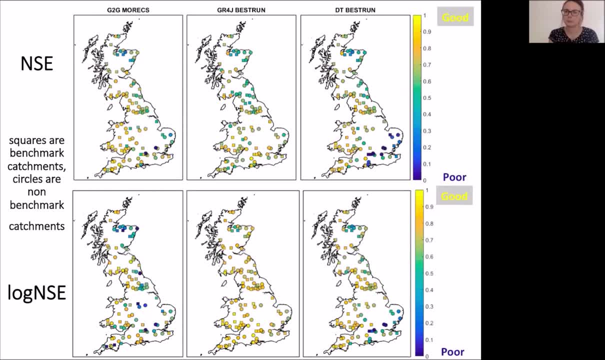 Again, just to pick up on the fact that you know, we do have some slight differences in terms of what models produce in terms of output, And on the bottom panel is log NSE. So this is more focused on the low flows. 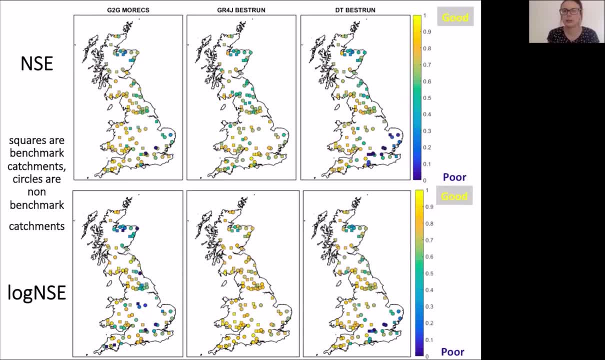 So, firstly, actually the models are doing really well overall across. you know a large proportion of the catchments in Great Britain. You know they're simulating a wide variability of hydrologic and climatic diversity and producing good simulations. However, there are a couple of key things. 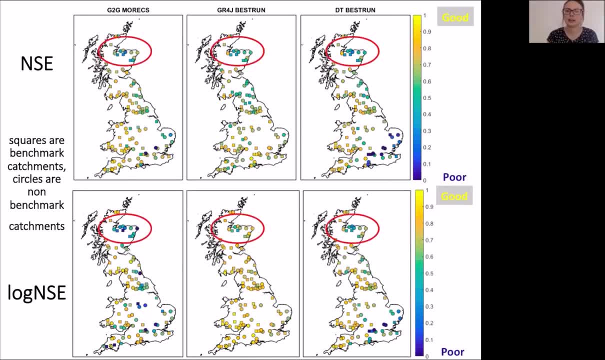 that we can really note from these plots. So, firstly all, the models tend to perform not as well in North East Scotland. A couple of reasons why we think this might be: it might be due to water storage and reservoirs or because of snow melt contributions. 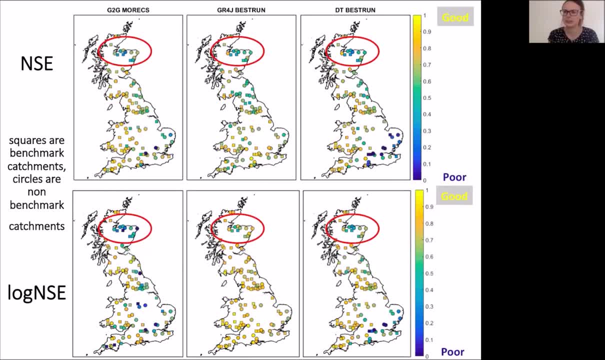 Currently, none of the models have a snow model in them, And this is something that we definitely want to look at in the future. Secondly, all the models perform better in the west of the country, So in wetter generally, wetter catchments. 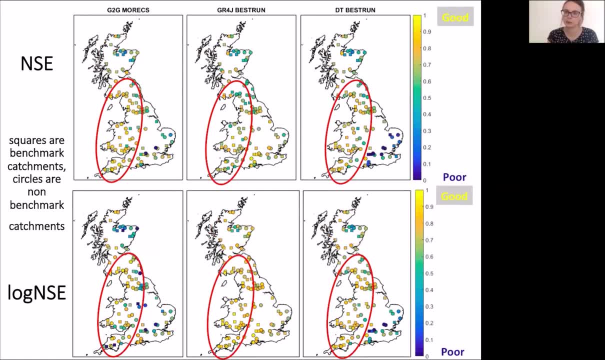 which isn't overly surprising, But the best model results are kind of found in the west of England and Wales And finally, the biggest model differences are really found in the southeast. So this is where a grid to grid and dynamic top model tend to struggle in terms of reproducing observed flows. 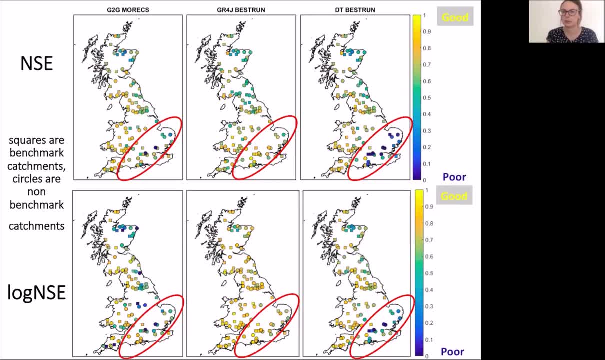 And actually GR4J does very well in these catchments. And if we delve into the model results a bit further, we can see that GR4J does very well in these catchments. We can see that if we look at the bias. 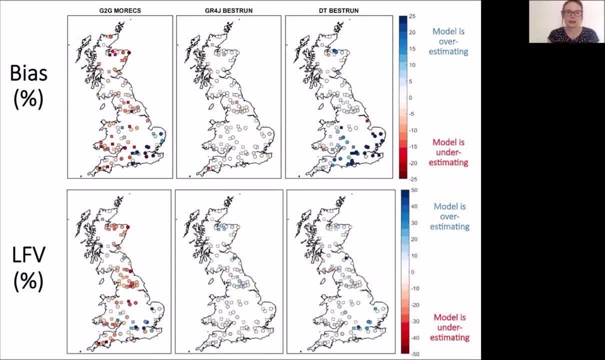 we can sort of see some reasons for this difference. So again, each of these, each of the points show a gauge and we've got bias sent in the top panel and low flow volume in the bottom panel, And here the blue color sends. 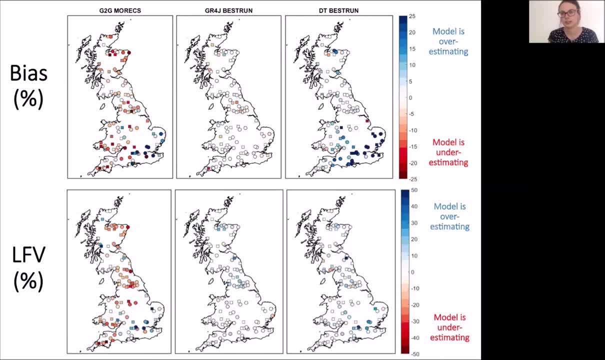 shows that the model is overestimating the water flows And the red color shows that the model is underestimating the water flows. So in the southeast can see that both grid-to-grid and dynamic top model are just too wet. We're producing too much. 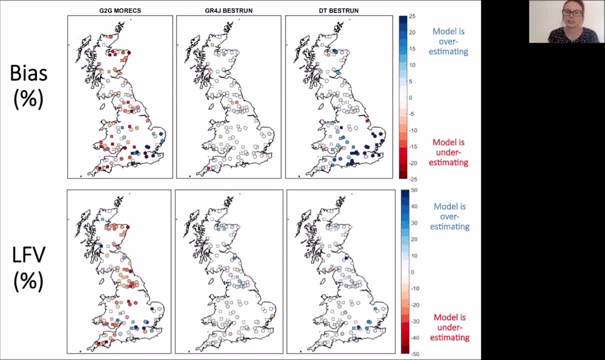 flow in our simulations compared to GR4J. Grid-to-grid tends to then underestimate the flows kind of in the west and the north of Great Britain. There are some really good reasons for this. GR4J has a parameter that you can calibrate that essentially defines intercatchment water. 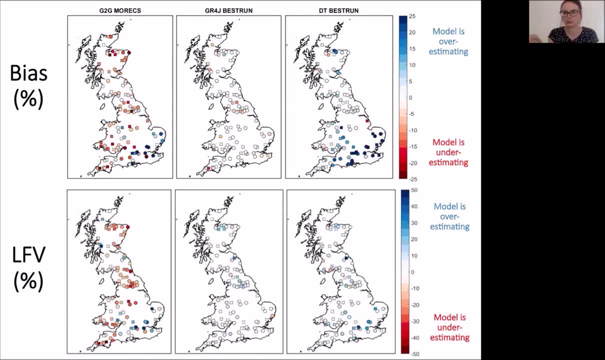 flows and essentially is a water loss or water gain from the model. They have a parameter that they can tune in the model. that essentially means they can lose as much or as little water in the time series as they need to be able to fit the flows. Dynamic top model and grid-to-grid. 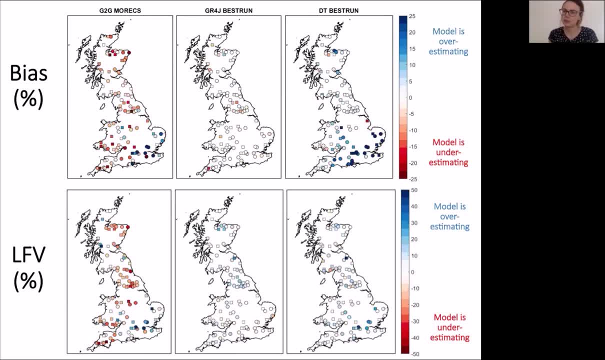 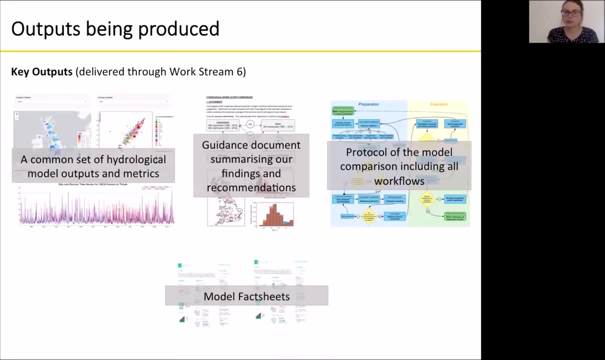 both maintain water balance and so essentially what's happening is we just we just don't have enough water loss from the model, given the rainfall inputs and the PET output. So this explains the differences, So the outputs being produced from this work. So we've produced a common set of hydrological model outputs and metrics. We're also currently 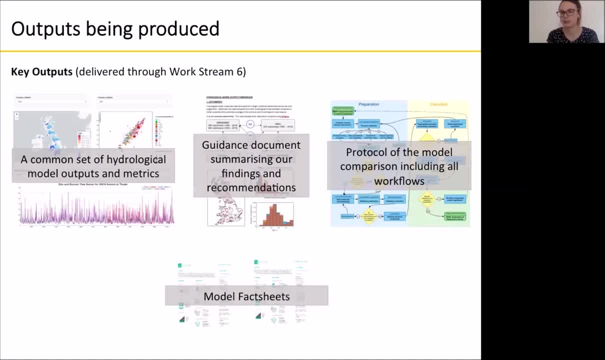 producing a guidance document summarising our findings and recommendations and a protocol. so this is a very complex model of the model comparison, including all workflows And some model fact sheets so that if you wanted to read up more in terms of what processes are in which models, or how they were calibrated or what input data they used, you could use these. 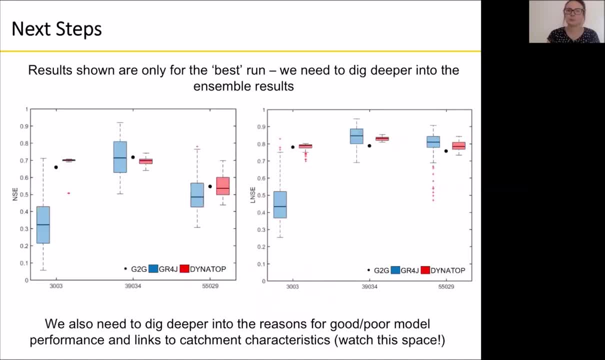 fact sheets to help answer those questions. However, we've still got a lot of work to do so over the next six months. really, what we're going to be doing is delving deeper into the ensemble, so the results I've shown you today are just simply for the best run. 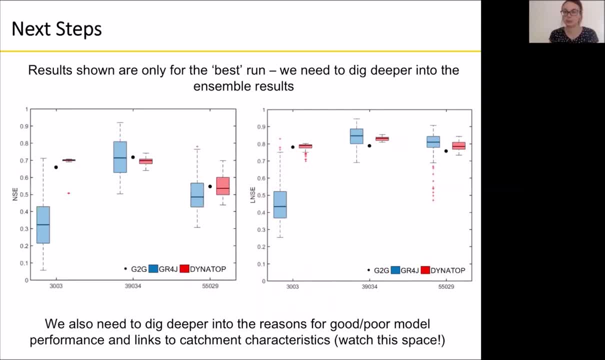 but GR4J and dynamic top model actually have ensembles of model simulations. So in the box plots below you can see three different catchments and the blocks plots essentially show the range of model results from the ensemble. In blue is GR4J, in red is dynamic. 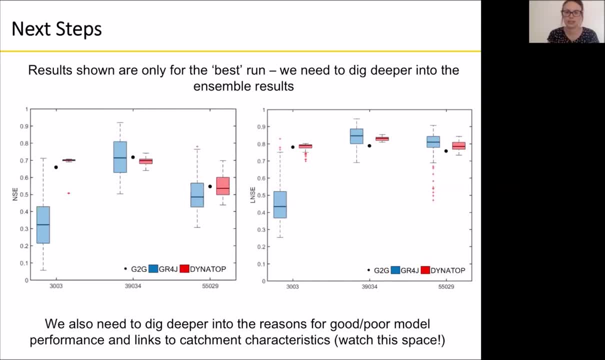 top model and then the dot is grid to grid. that has one model simulation. We also need to dig deeper into the reasons for good- poor model performance and link this better to catchment characteristics. so I gave a few reasons earlier on as to why we were seeing good or poor model. 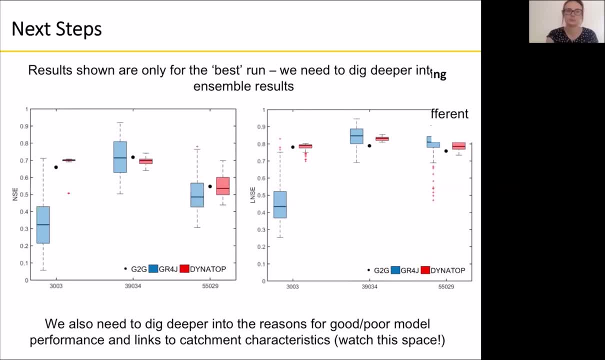 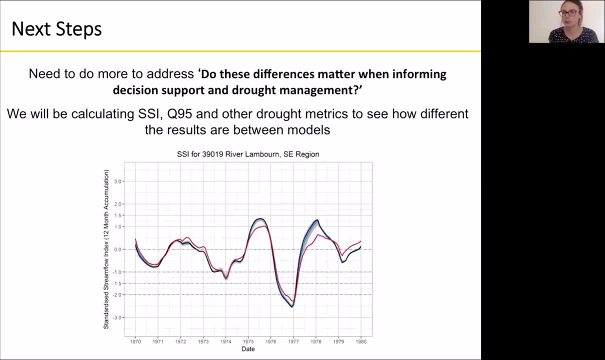 performance, but we need to delve into this further. The final step of this project is: do these differences matter when informing decision support and drought management? So okay, we see that our model performances are different in different places. we have different evaluation metrics, but actually how? how does this matter when? how much does this matter? so,